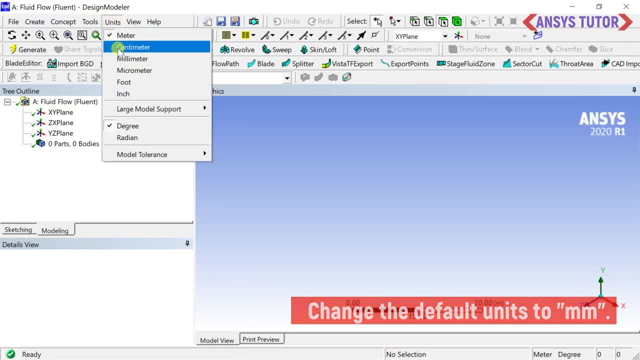 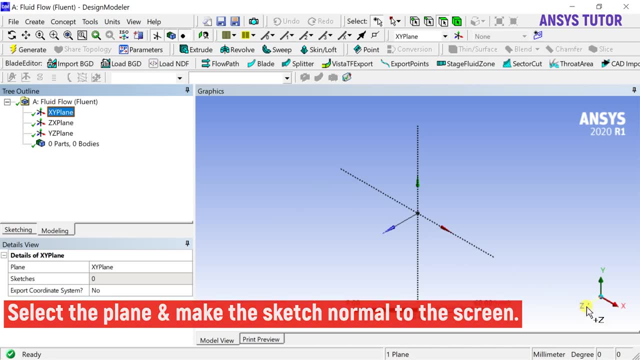 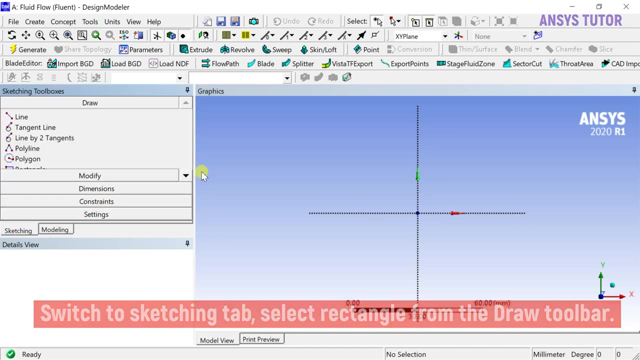 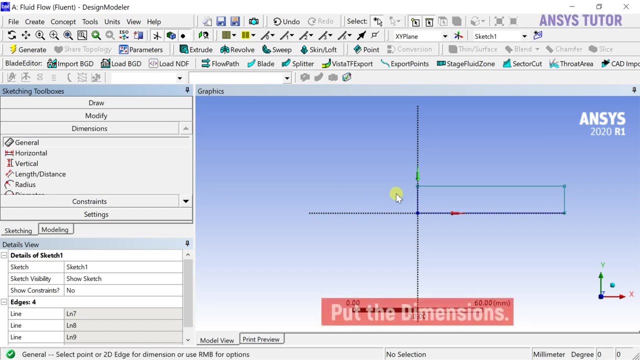 Change the default units to millimeter. Select the XY plane. click on the Z to make the sketch normal to the screen. Switch to sketching tab. Select the rectangle from the draw toolbar, Place this+. Find the 3D image in the lower right of the document. 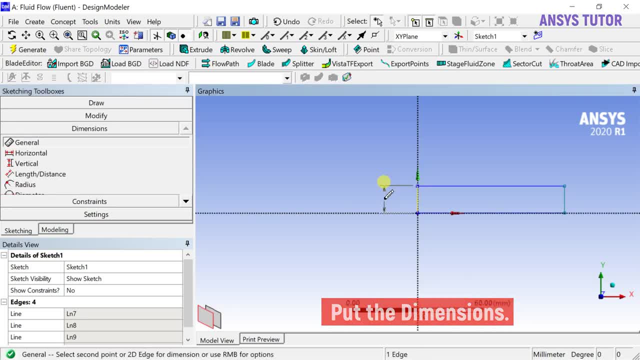 Here I'll retain the image. Put dimensions in Bueno hard to the rectangle. Set the upper right's, Here's the U, lower left, the zero andIZ model. Please again make adjustments to the list. Use the place number to select an image. 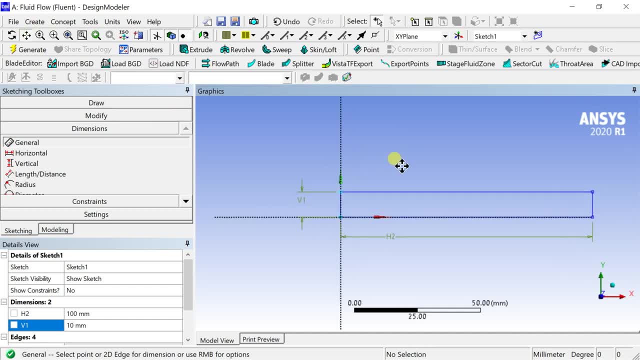 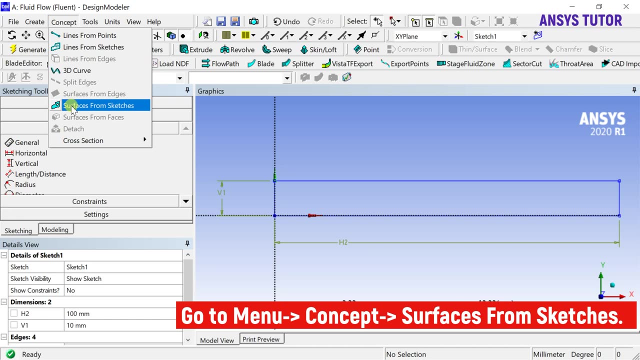 But if you press button arrow you will die to the result. Now the sketch is complete, We need to convert this sketch to a 2D geometry. For this we need to go to the concepts menu. here we can get the option surface from sketches. 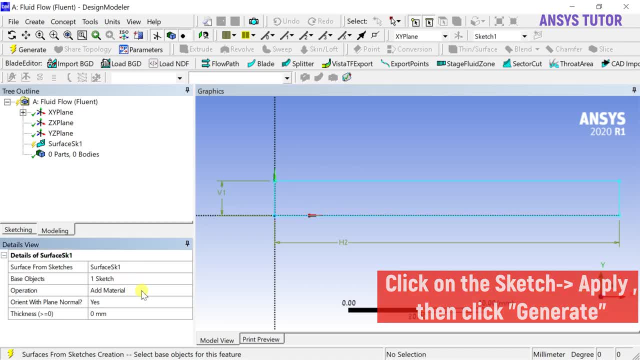 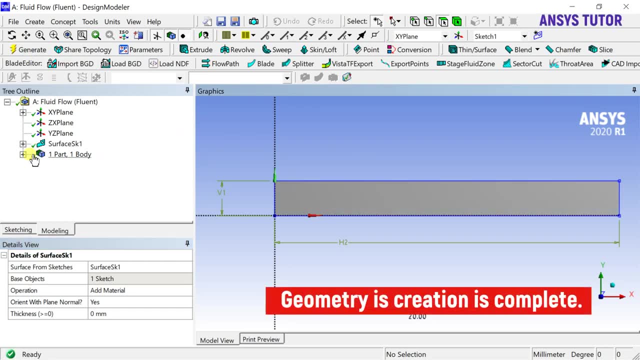 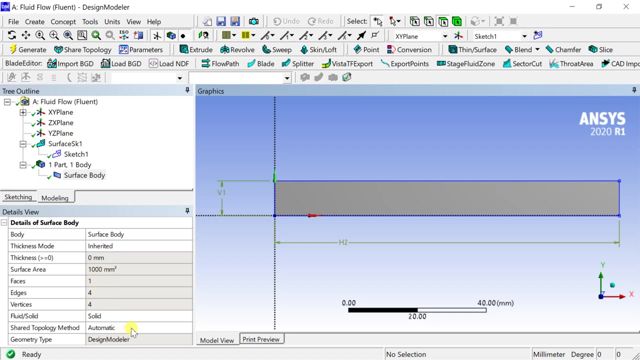 Using this option, we will convert the sketch to a 2D geometry. Click on the surface body from the tree outline Now. the details of the surface body table appears in the left corner In this table. change the body type to fluid, So the meshing software will mesh it as a fluid domain. 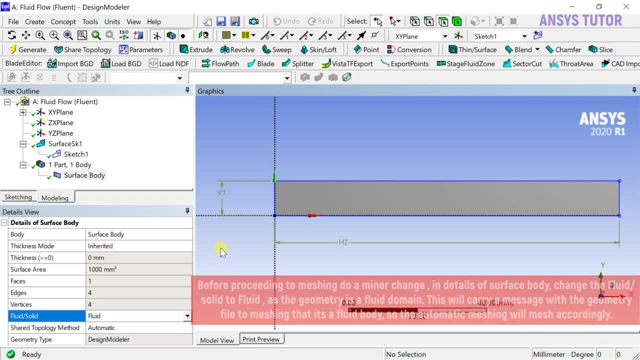 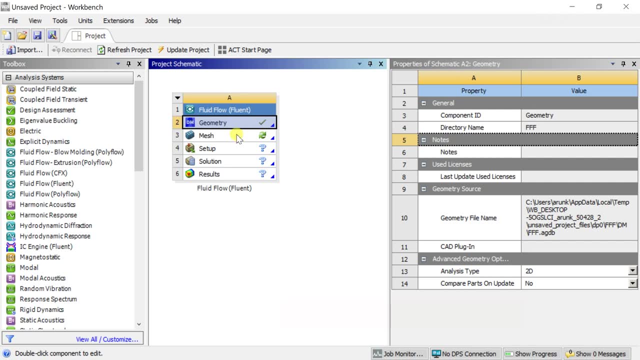 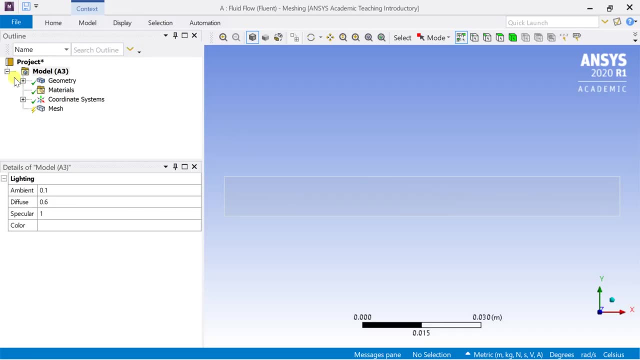 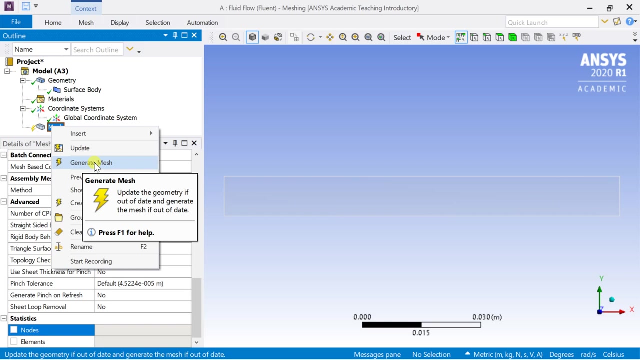 Ok, Now proceed for meshing the geometry. Open the meshing workbench window. By default, ANSI's meshing has set some default mesh sizes for this geometry, So let's generate the mesh using default mesh settings. Ok, Let's change the general mesh size to about 3600. 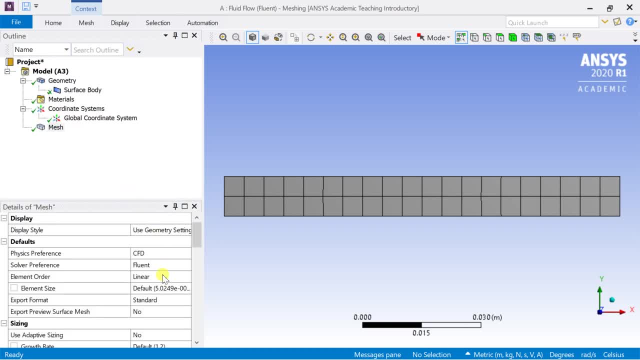 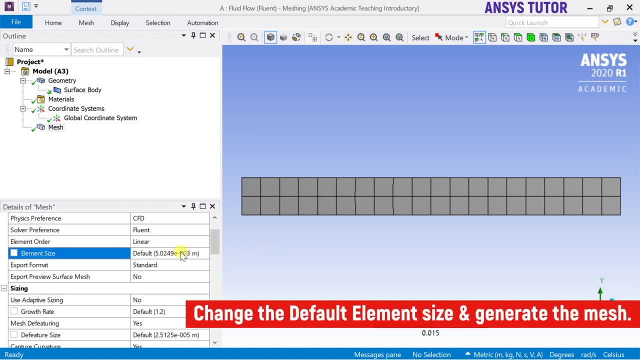 This is the default generated mesh. Now we gonna modify the default mesh setting to further decrease the mesh size. Let's change the default element size and generate the mesh. OK, Now we can create a new mesh. Make sure that the border is in the center. 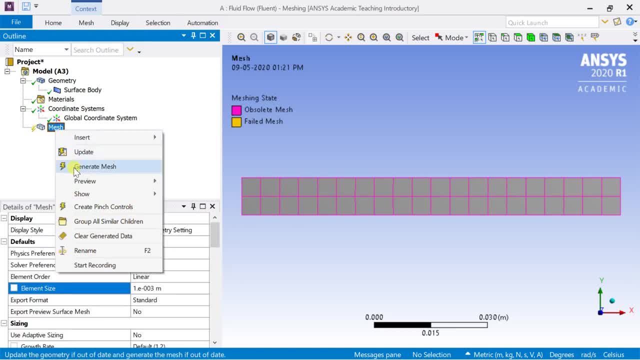 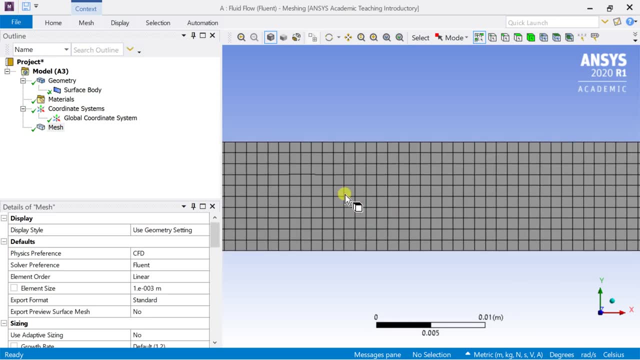 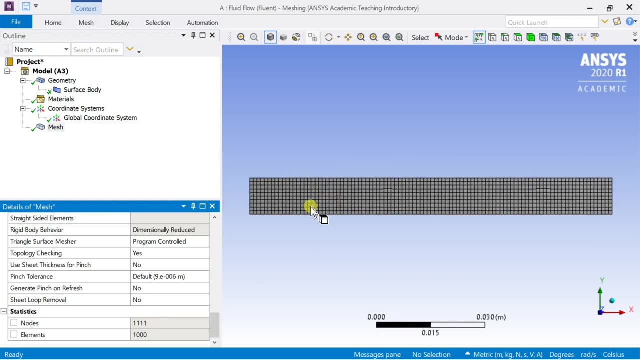 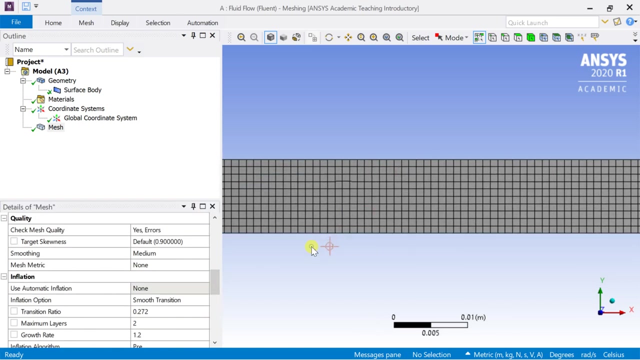 To do this, we need to change the element size Now. set the border to 2200.. Ok, Now the mesh will be generated. Let's change the default element size and generate the mesh. Ok, Check the mesh statistics to see the generated nodes and elements. 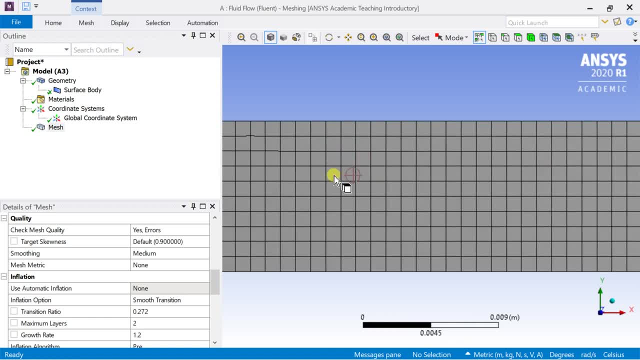 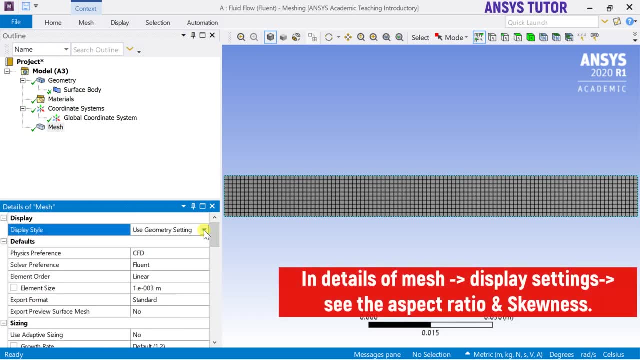 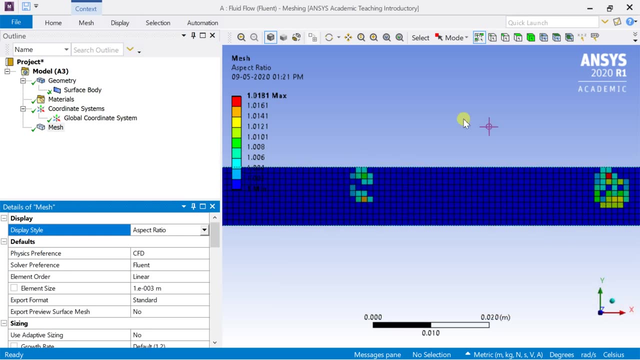 Let's check the aspect ratio of the generated meshed cells. For this you need to select display style and details of mesh. You can see the meshed cells are not distributed properly in some regions. for this we need to change another setting, that is adaptive meshing. 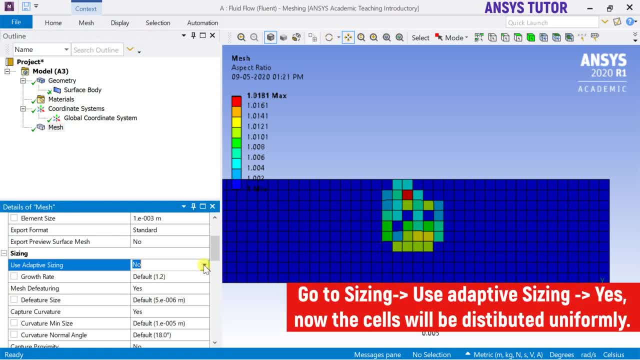 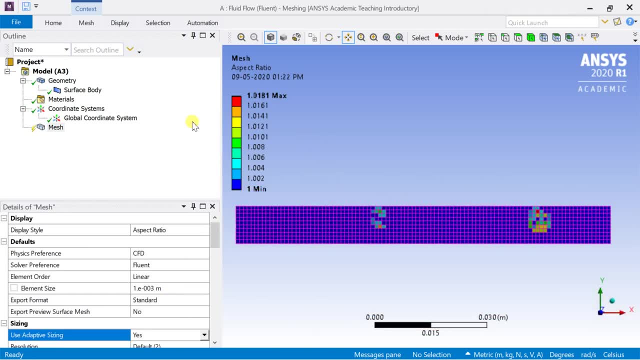 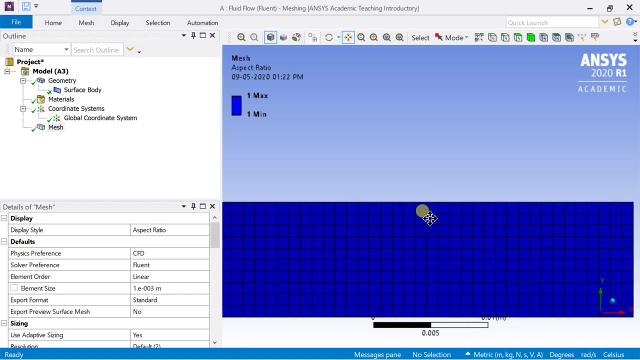 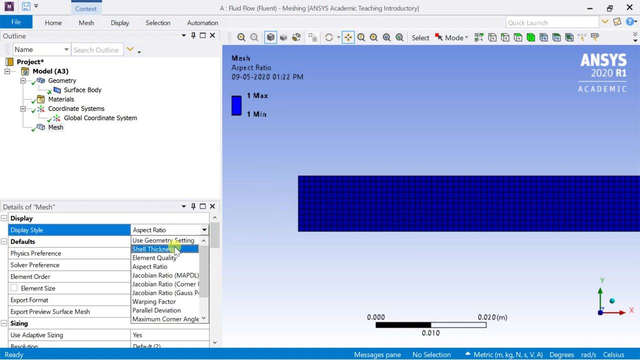 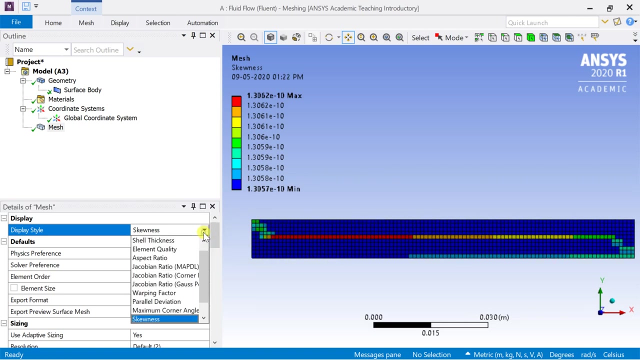 We need to turn on adaptive sizing to distribute the mesh uniformly throughout the geometry. Now all the meshed cells are distributed uniformly. It now a structured mesh. You can also check the skewness of the meshed cells using the display style. We would discuss more about the meshing and how to check the quality of the mesh and its 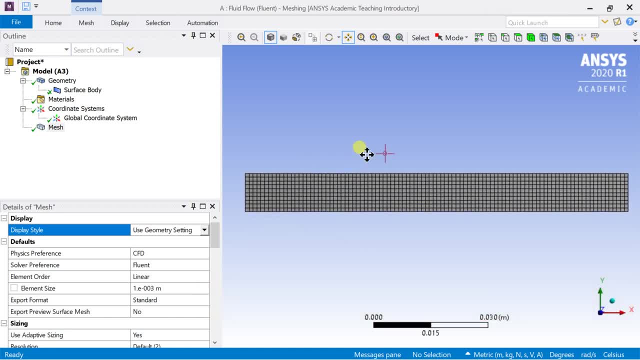 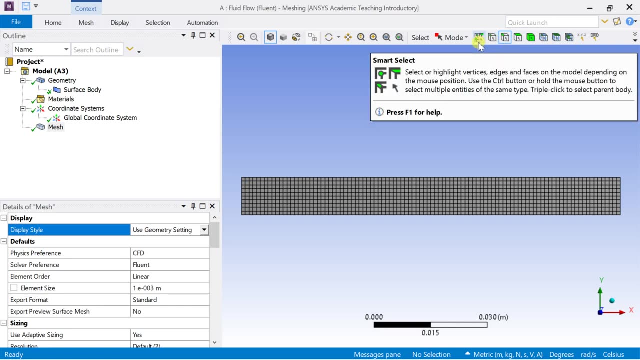 importance in our upcoming videos. Now we would select the boundary, to name it. for this, we need to choose the selection tools. Here are the selection tools: Vortex Selection, Edge Selection, Surface Selection and Body Selection options are available here. Now let's check the selection tools. 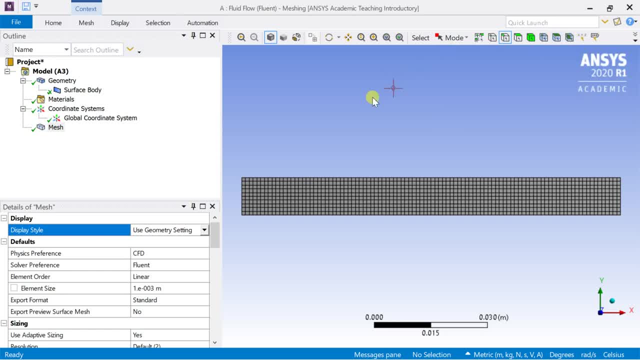 Here are the selection tools: Vortex selection, Edge Selection, aders. From this, select the Edge Selection option and select the edges in the geometry. Select the edge, Then right click, then select Create Name Selection from the menu. now put a name for. 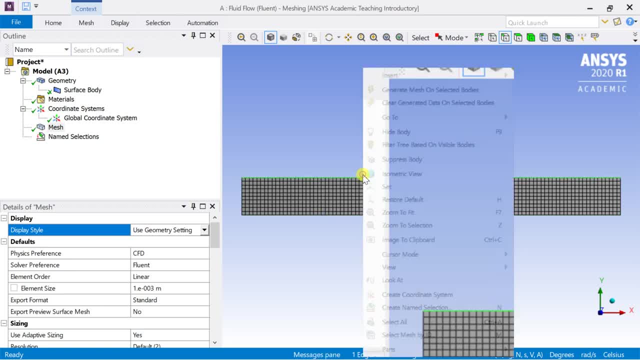 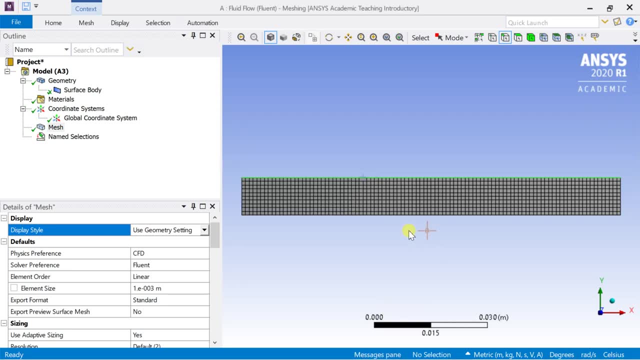 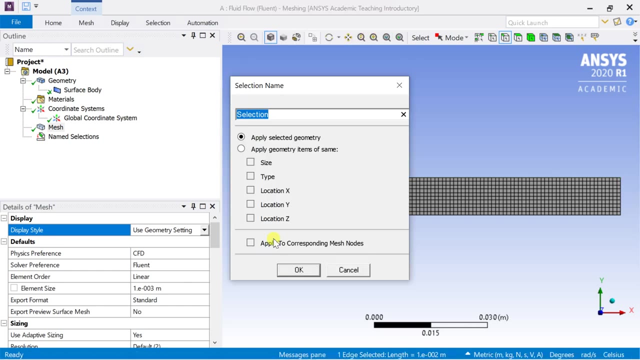 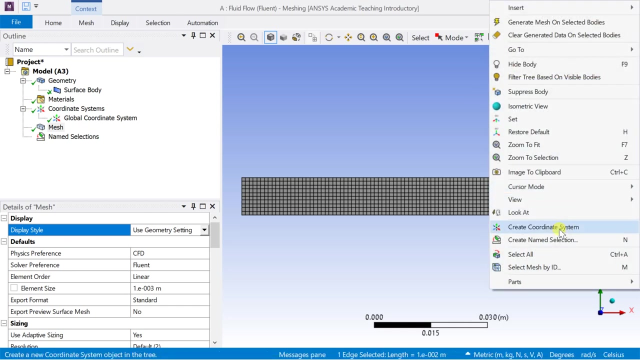 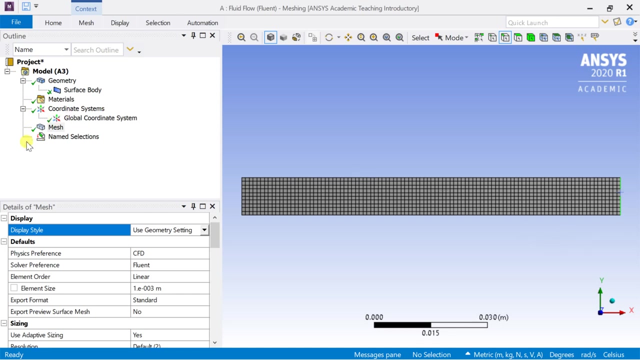 the boundary surface. We had denoted the bottom edge of the rectangle as axis. as it's an axisimetric problem, similarly name the other boundary surfaces. Right click the surface. All the named boundaries are listed in the tree outline under Named Selection. 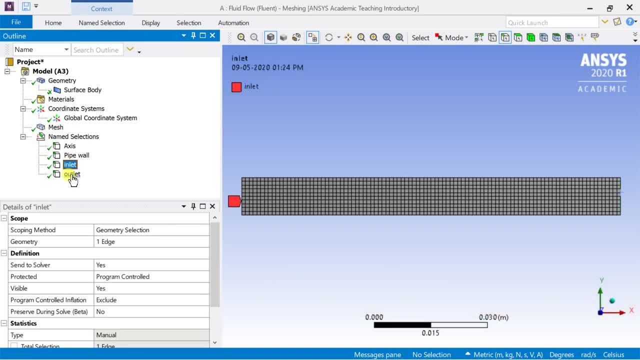 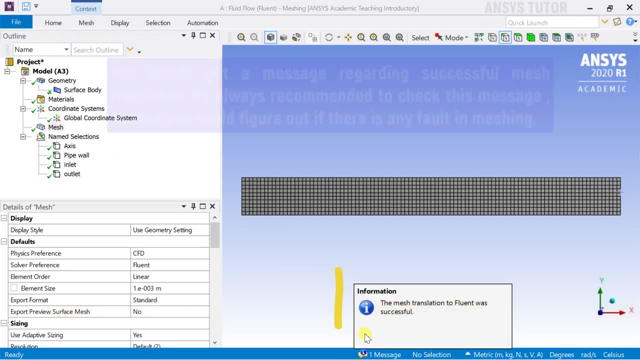 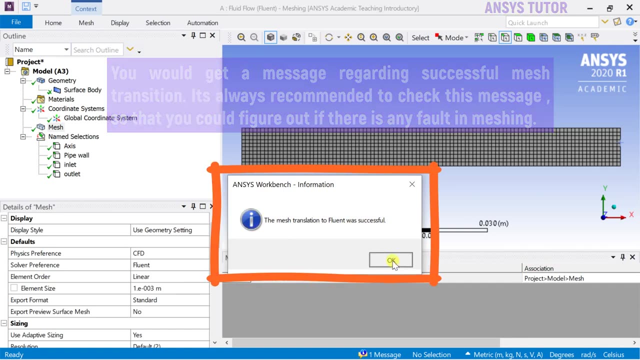 You should cross-check these named selections once, As if a boundary is named twice, then it might cause error on updation. Right click on Mesh and select Update. it will update the generated mesh with the Fluent CFD solver. You would also receive a info message regarding this. 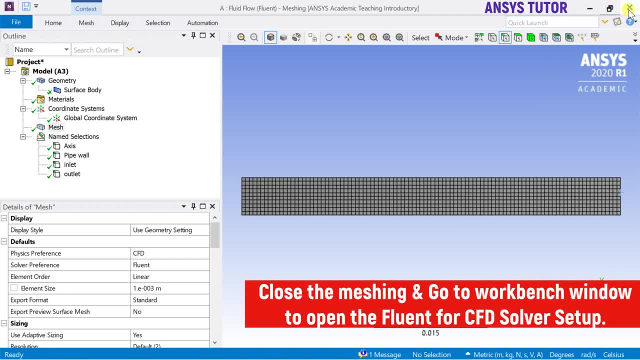 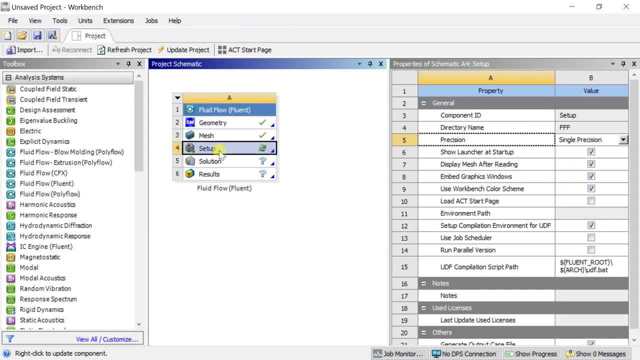 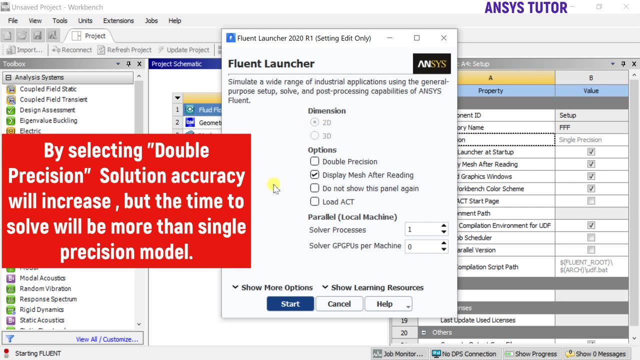 Close the meshing and go to Workbench window to open the Fluent for CFD solver setup. Right click on Setup and then select Edit. Now a Fluent Launcher window will appear. it will ask regarding whether you want to set single precision or double precision. solver number of CPU. 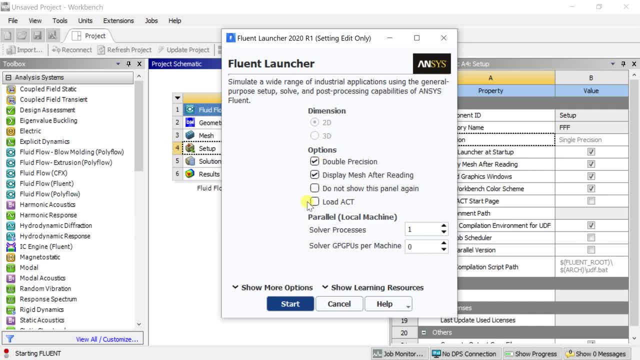 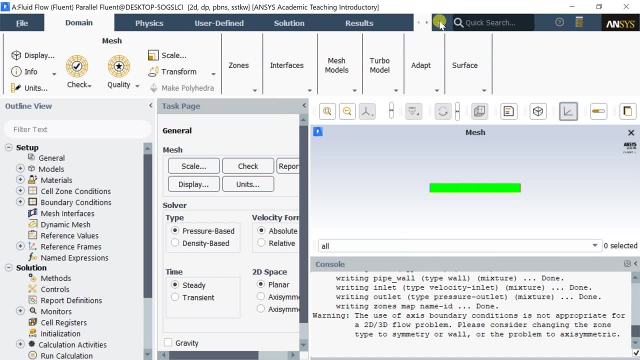 processor to employ series and parallel solver, etc. We will discuss more regarding this in our upcoming videos. For the current simulation, select the double precision model and press OK. This is the ANSI's Fluent solver window. here we would put all the boundary conditions. 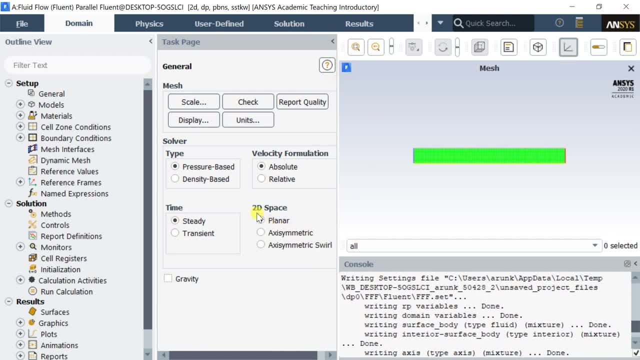 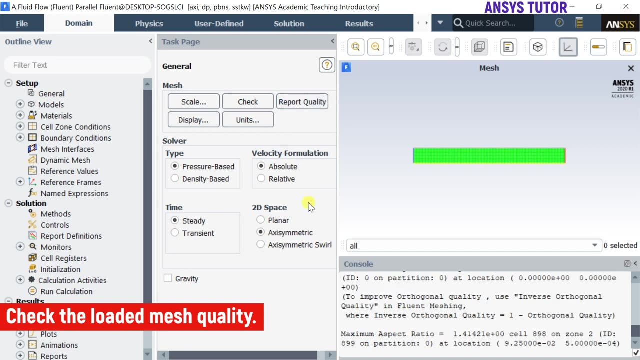 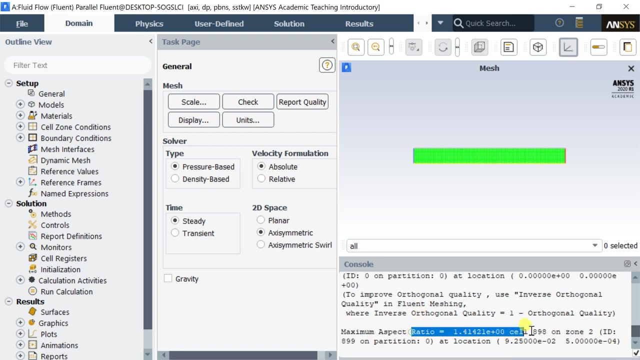 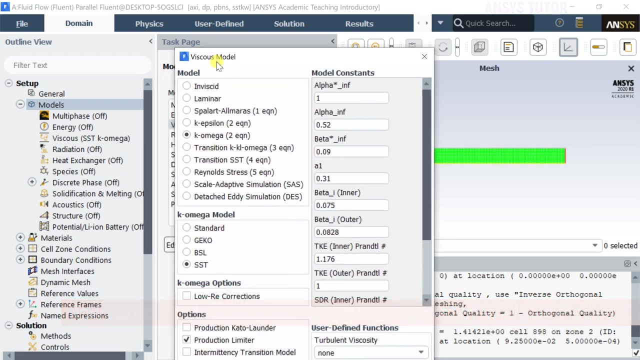 and will do necessary setups, which is required for the analysis, As it's an axisymmetric analysis, so you need to select axisymmetric 2D space. Check the loaded mesh quality. Select the required flow model from the list of available models. 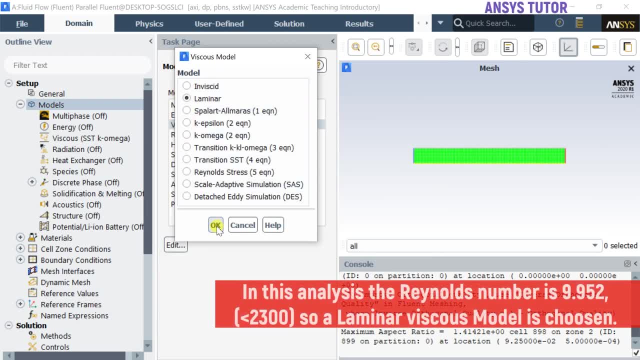 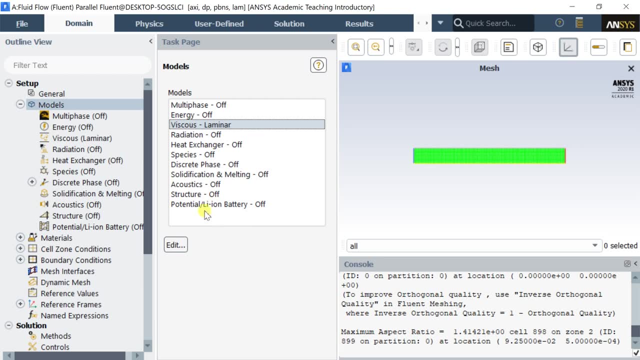 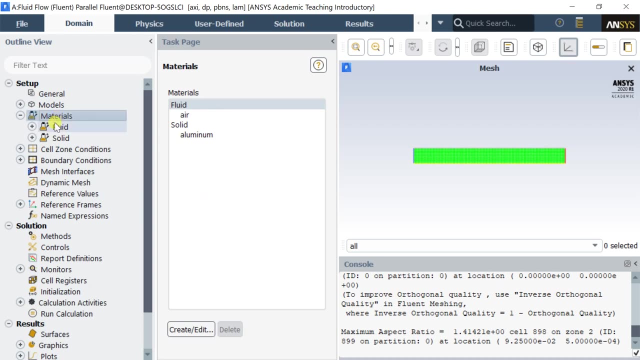 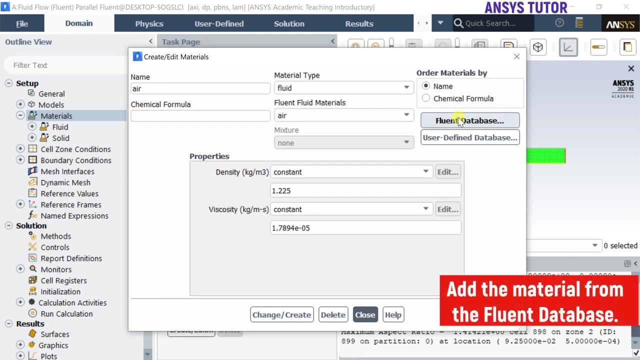 In the current problem The Reynolds number is 9.952, which is less than the Reynolds number 2300 for pipe flow case. So a laminar, viscous model is selected for this analysis. Now load the fluid material from the Fluent database. 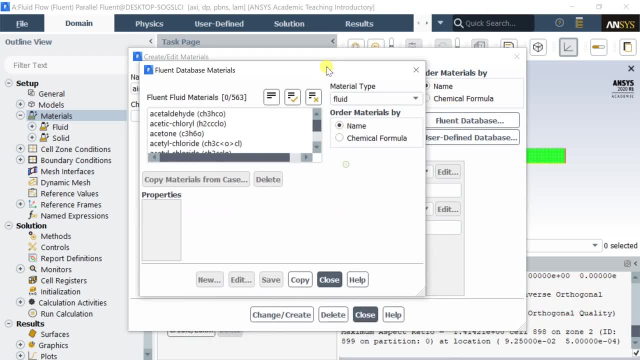 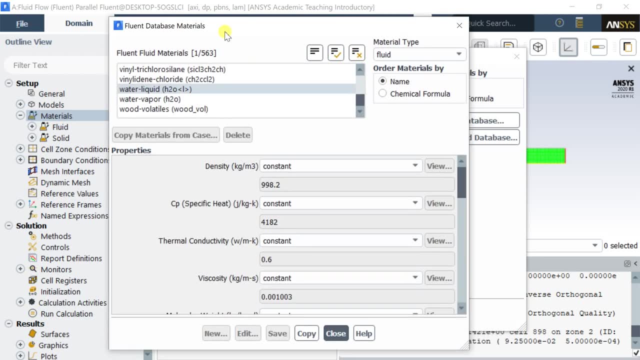 You could also change the material properties as per your requirement. for the current simulation, let's take default water as the fluid. As you can see, the flow is very smooth To add the fluid material. you can only add the necessary material properties of the. 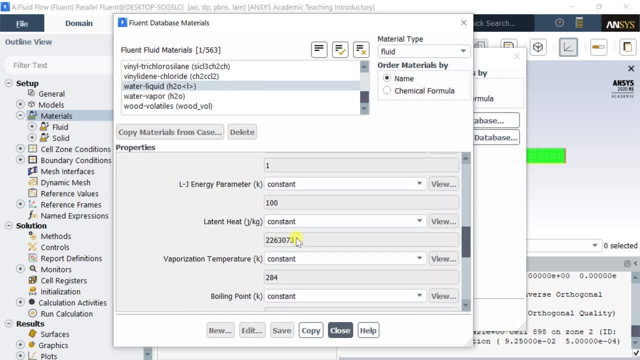 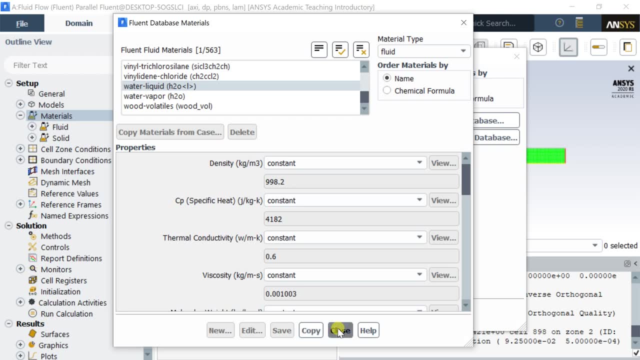 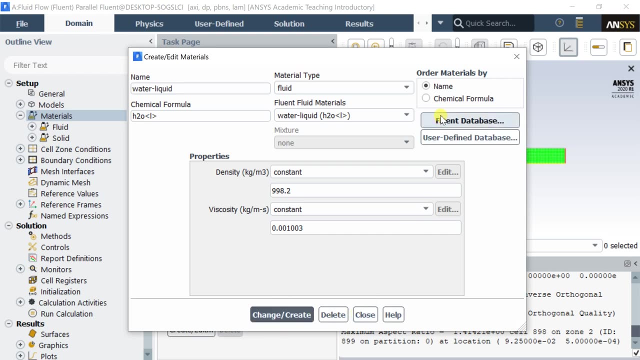 selected model And this is the sample of the fluid material. You can also add the solid material. The flux is based on the fluid material in the fluid. The flux is based on the fluid material And this is the sample of the fluid material. 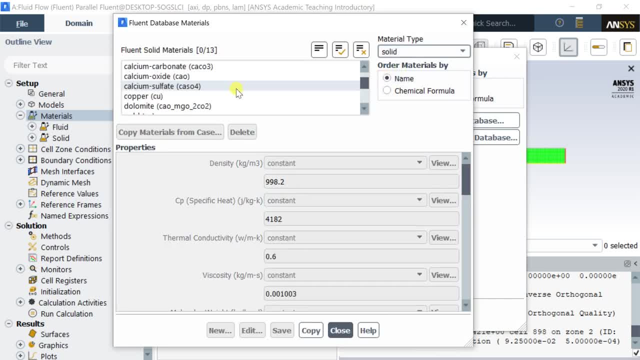 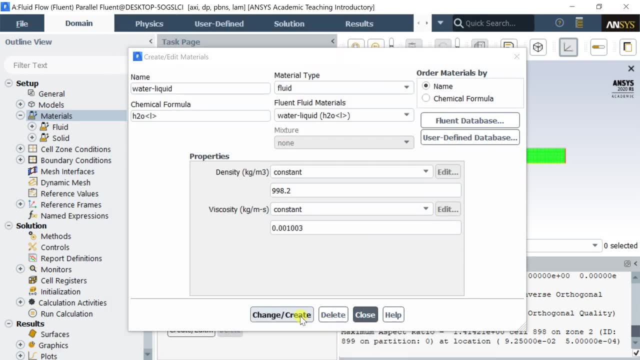 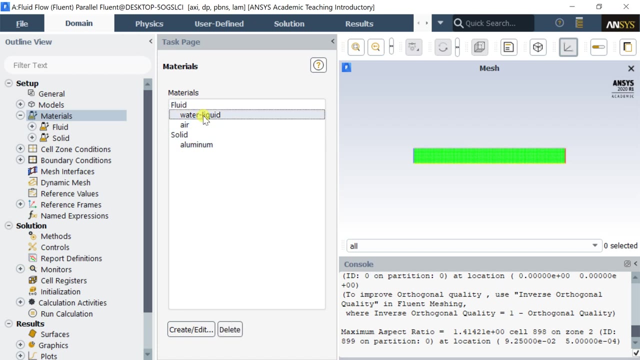 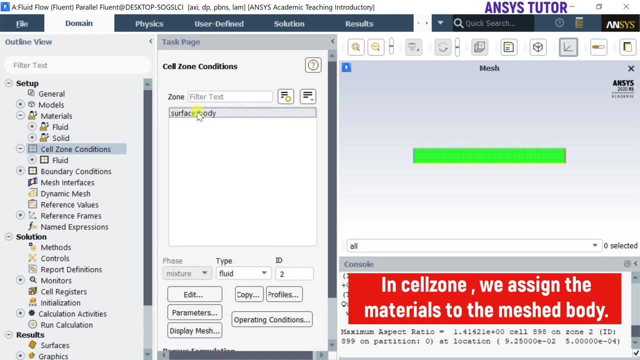 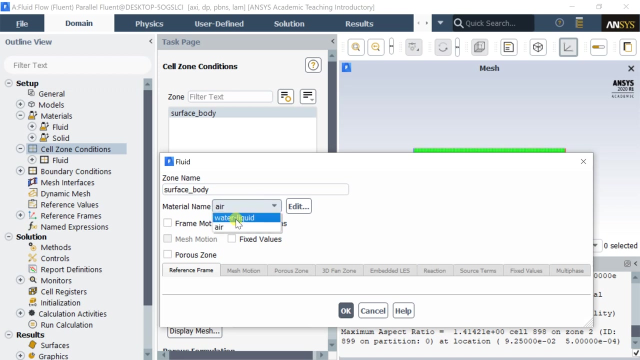 So you have to add as much as you can. Now let us begin the analysis. Thank you very much. Thank you. Solid materials from the Fluent database. by selecting material type to solid, Now assign the material to the fluid domain meshed body. 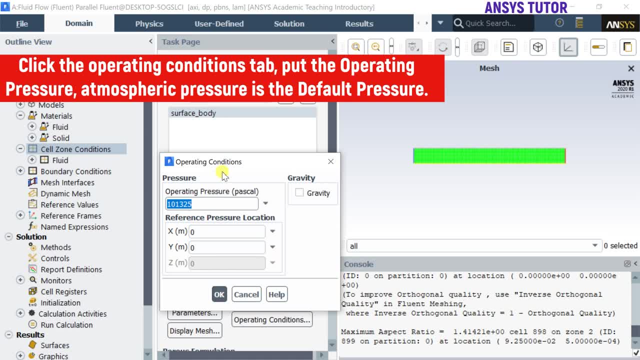 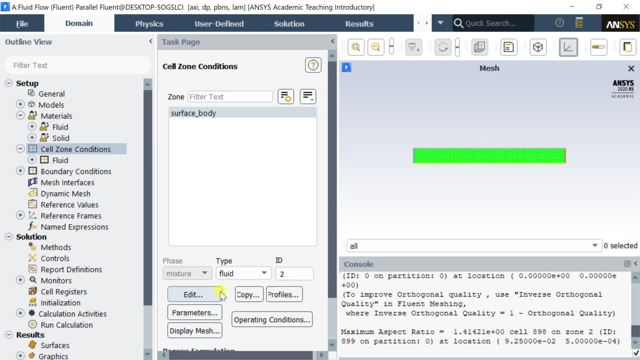 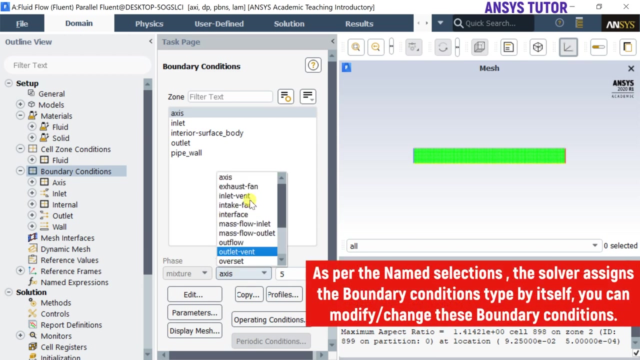 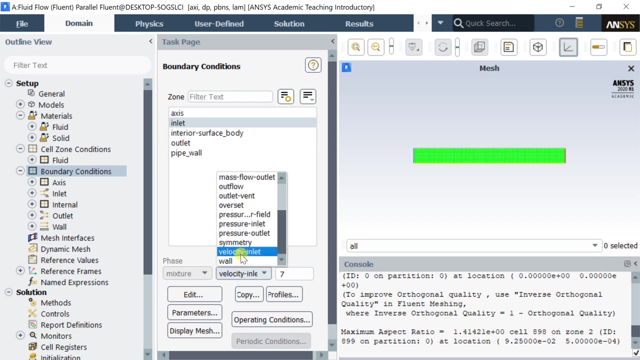 Click the operating conditions tab. put the operating pressure. atmospheric pressure is the default operating pressure. Switch to boundary conditions. select the boundary and put the required boundary conditions As per the name. selections. the solver assigns the boundary conditions type by itself. you can modify, change these boundary conditions. 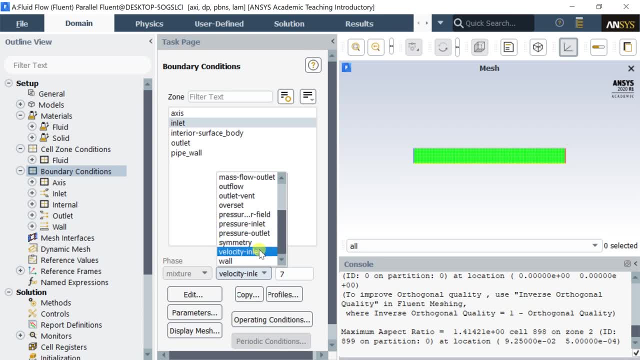 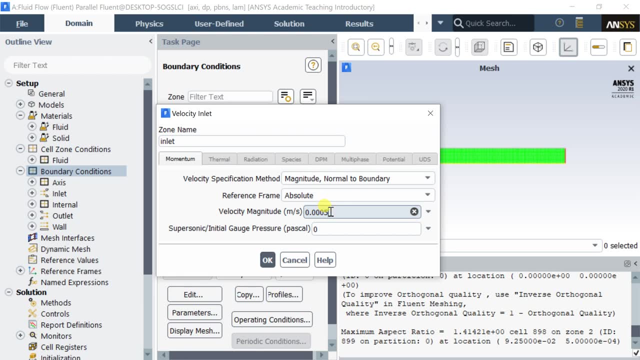 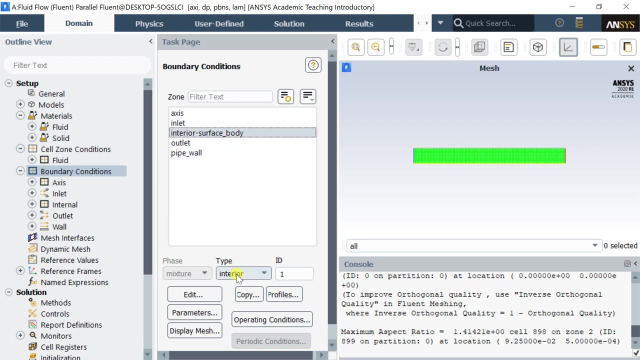 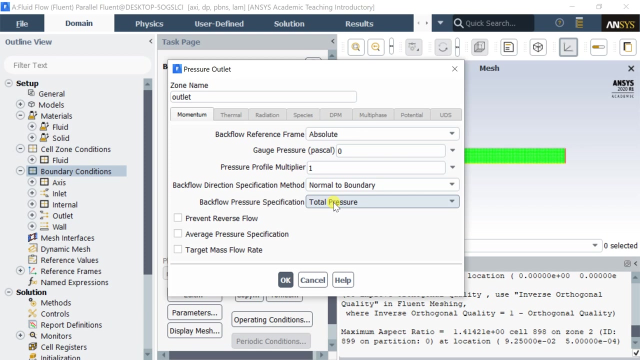 Select velocity inlet boundary condition. at the inlet end Put the inlet velocity of 0.0005 meter per second. Press ok. This boundary has been created by the solver, so no need to do any changes to this interior. Keep the default pressure outlet boundary type for the outlet boundary. 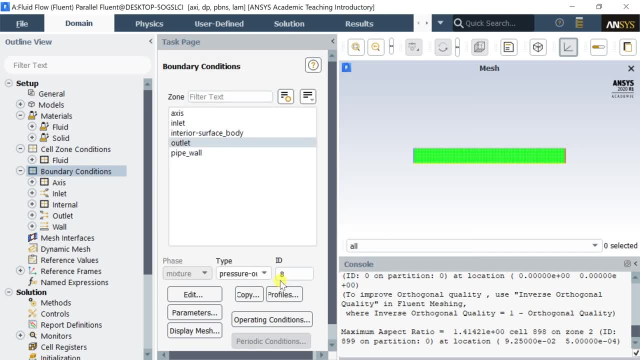 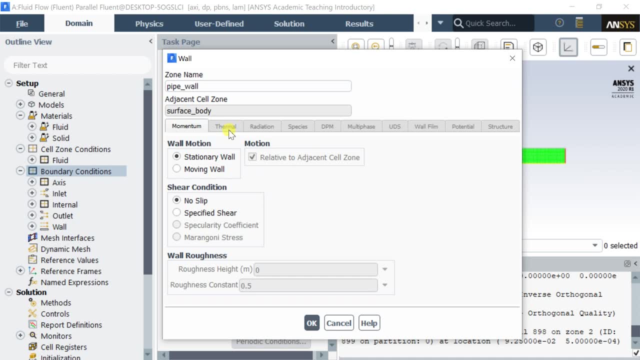 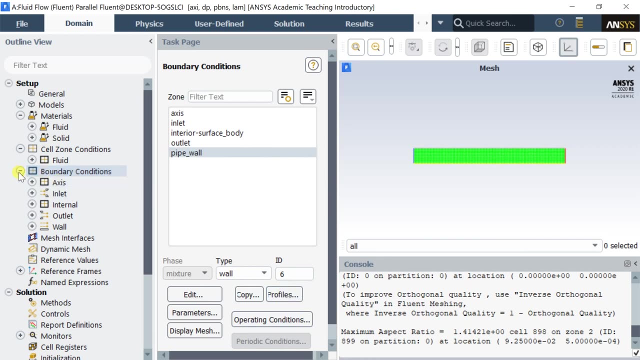 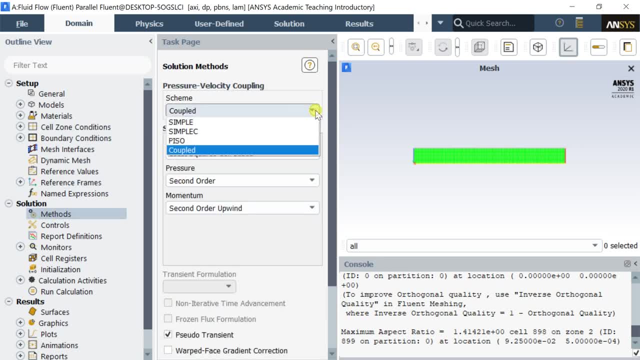 Just click, do more and look for more solutions here. just next: multimodal insulator. If you are using your computer, this system may contribute to cooperation, but for scheme quite the less. you will need solution easy to solve it. Now go to solution methods and select simple in the pressure velocity coupling scheme. 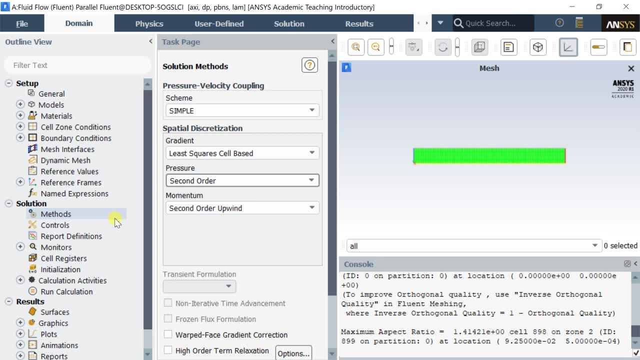 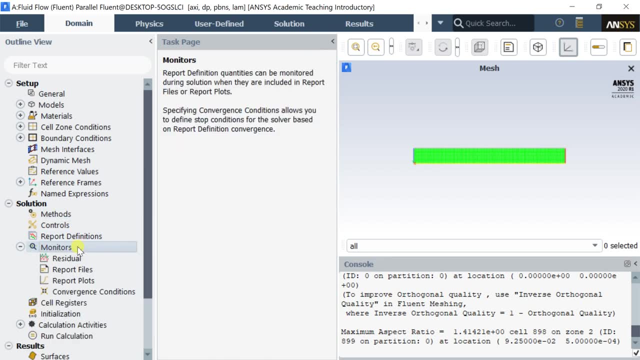 Simple defined is the semi implicit method for pressure linked equations. It means to instruct the solver to use simple algorithm to solve the numerical problem. To know about the details about how this algorhyton works, see the links in the descriptions. Now go to Monitors. select the residuals. decrease the residuals up to 10. to the power. 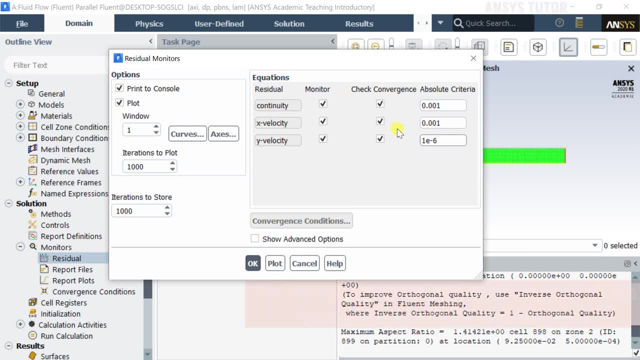 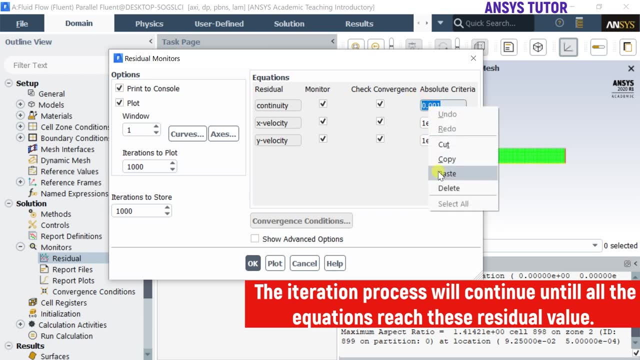 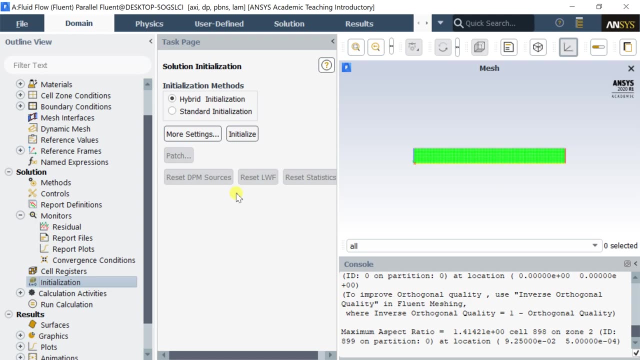 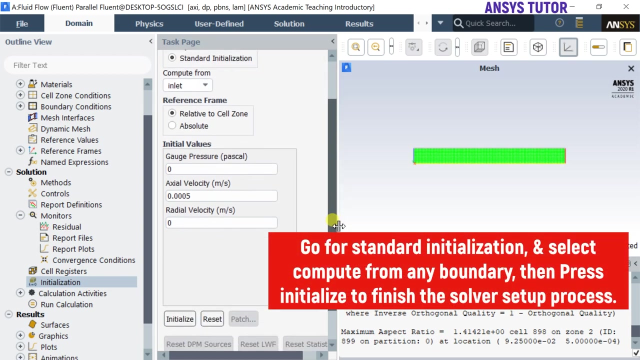 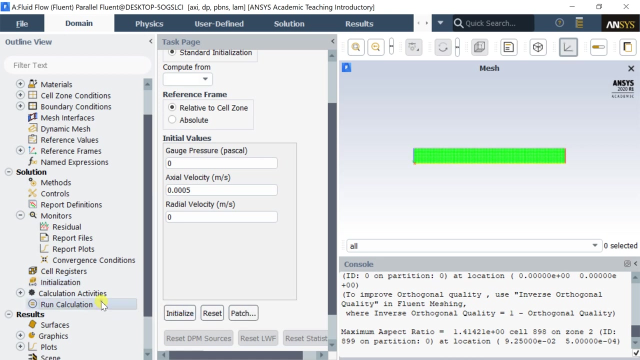 minus 6 for a better solution. accuracy: The iteration process gonna be continue until all the numerical iterations achieve this residuals value: Press OK. Click on Initialization. Select the standard initialization. Select Compute from any boundary. then press Initialize to finish the solver setup process. 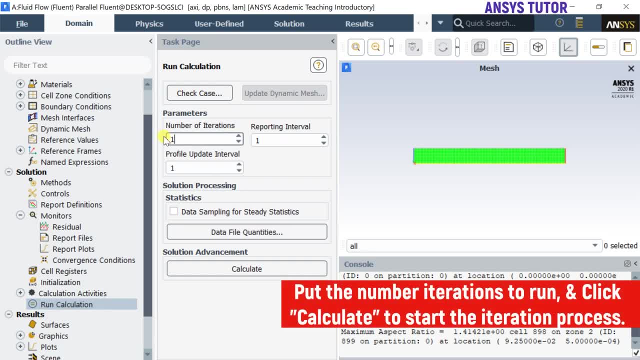 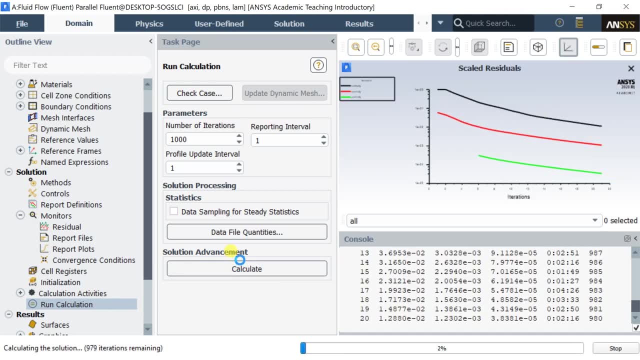 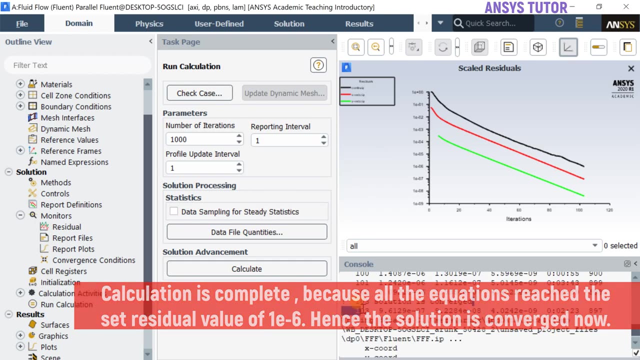 Click on Run calculations, Set the number of iteration to Run and start the iteration process by clicking on Calculate. Calculation is complete now. this is because all the numerical equations reached the set residual value of 10 to the power minus 6.. Hence the solution is converged now. 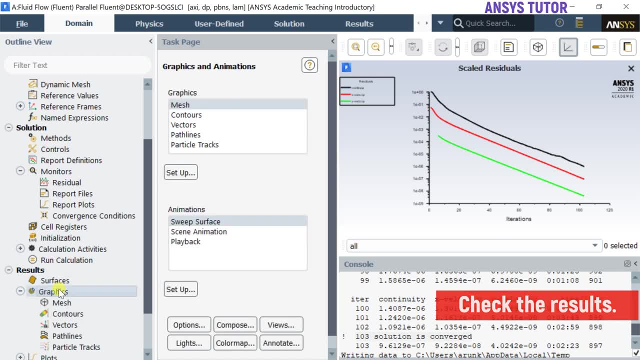 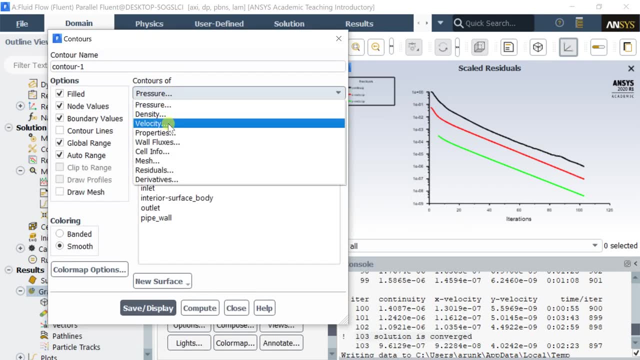 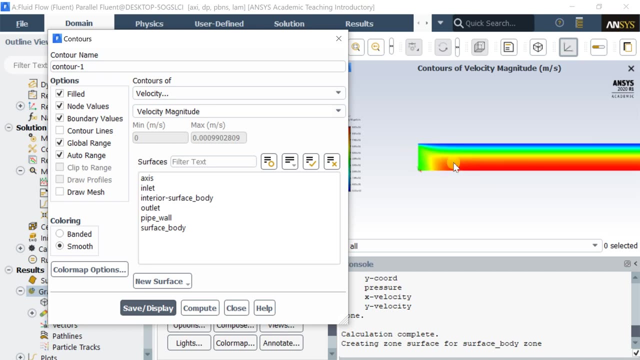 Now check the results. See the variations of velocity as a form of a contour. It can be seen that the velocity is maximum at near the central axis and decreases towards the pipe wall. As the velocity decreases towards the pipe wall, the velocity decreases to the pipe wall. 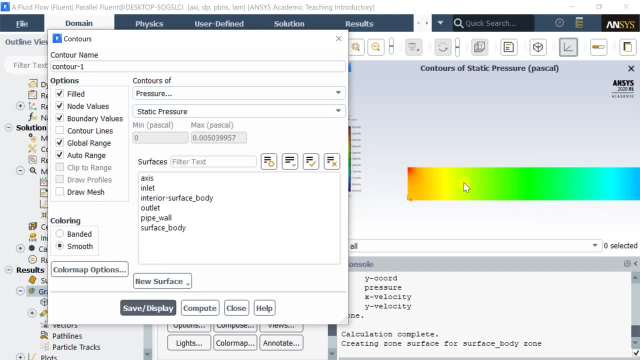 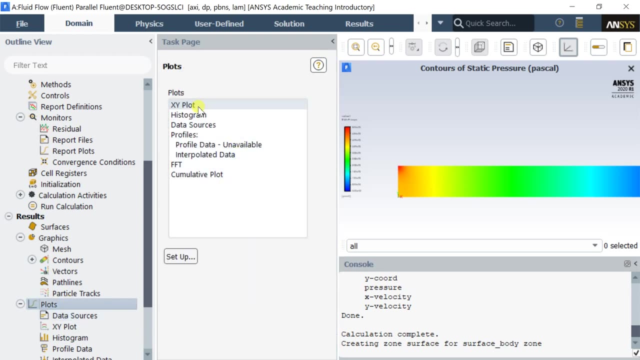 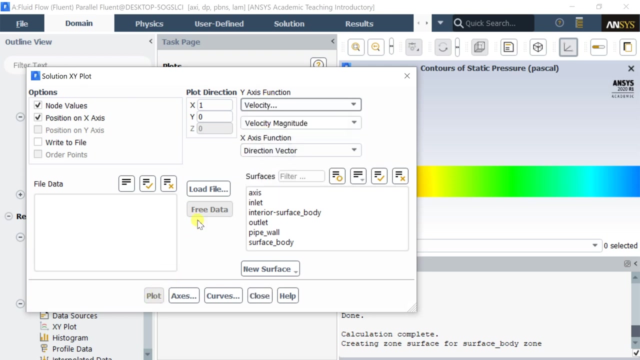 Similarly check the contour for pressure. Let's check the velocity variations along the central axis. for this, go to Plots. select XY plot. Select velocity in Y axis: function and direction vector. in X axis: Select the axis and click on iso. 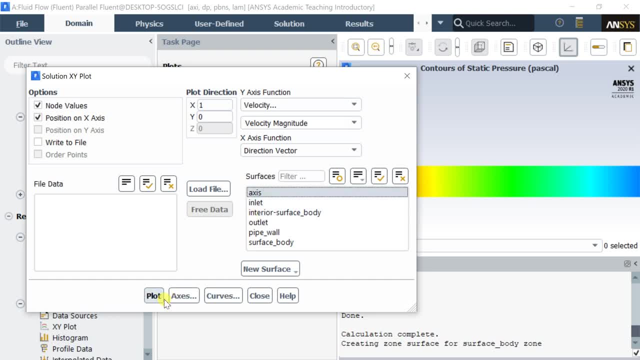 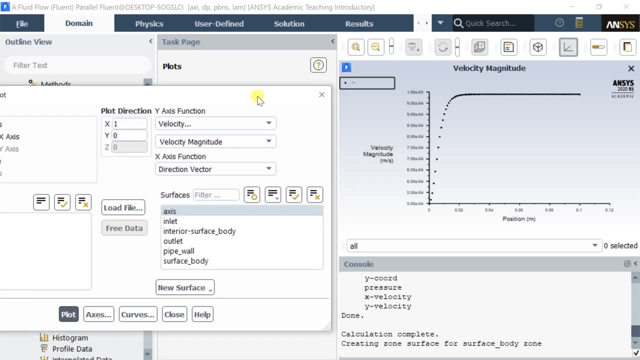 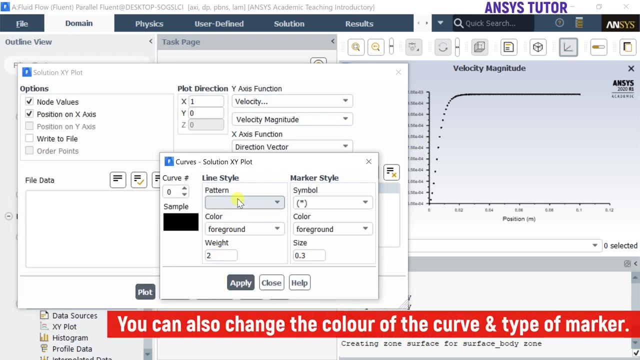 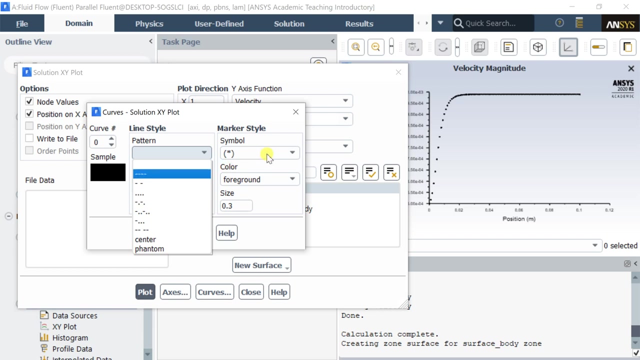 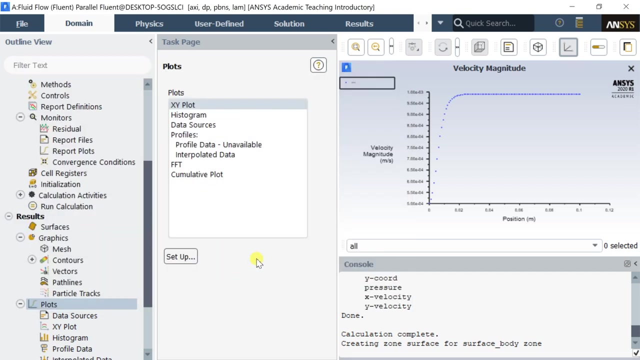 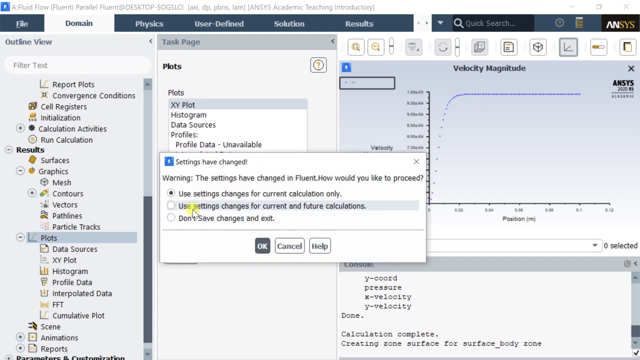 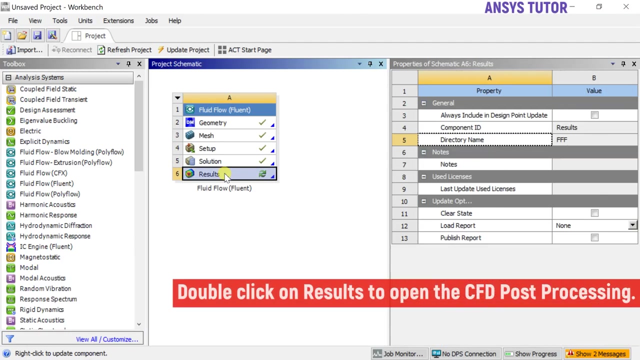 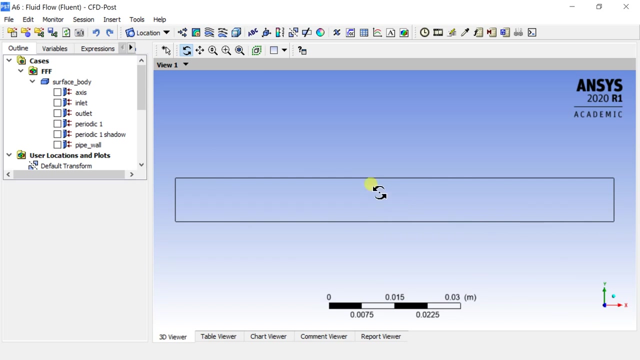 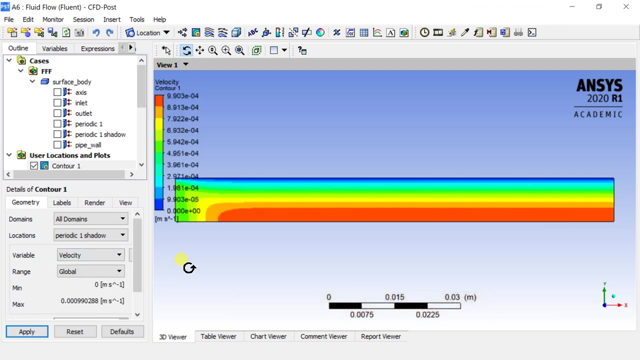 Select the center axis. Select X and Y axis function plot. You can also modify the color of the curve and type of marker for this plot. Now close the meshing and proceed for CFD post processing. This is the ANSI's CFD post processing workbench window. Insert a contour to observe the velocity variation. We would also create the contour for the full pipe body. 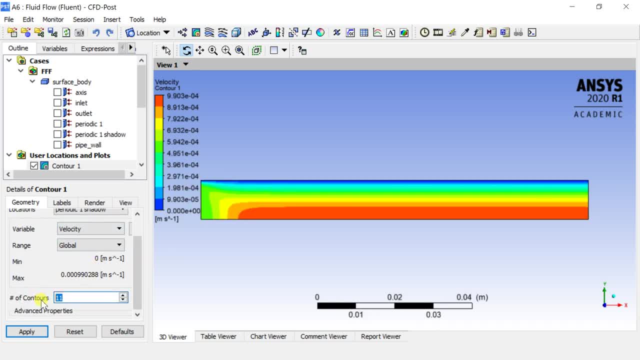 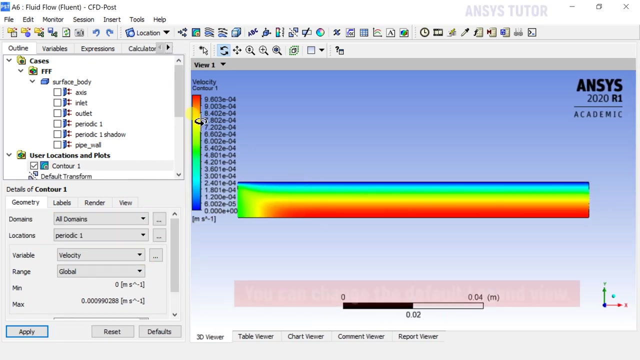 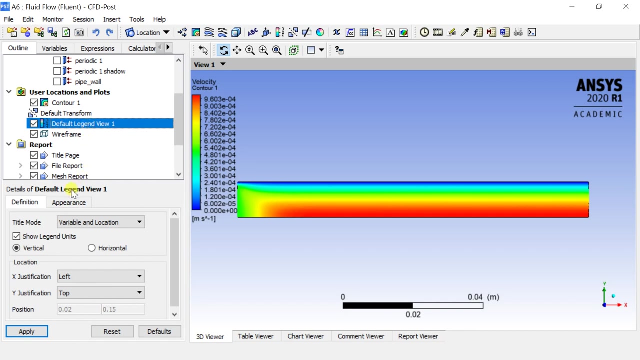 This denotes the color bands for the contour. For more number of color band, you can increase the number. You can also modify the default legend view. The entire page is cut out. Select your left new CTRL Stunden assumed value from these 3 options to modify it. 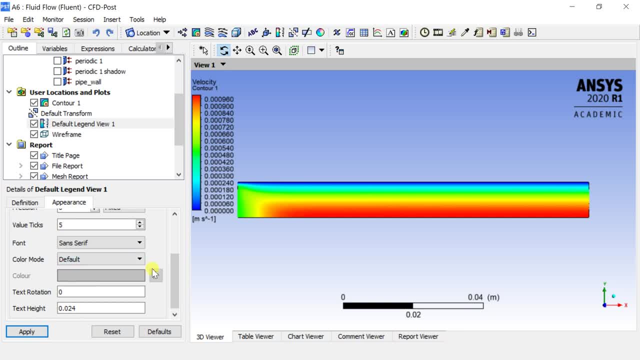 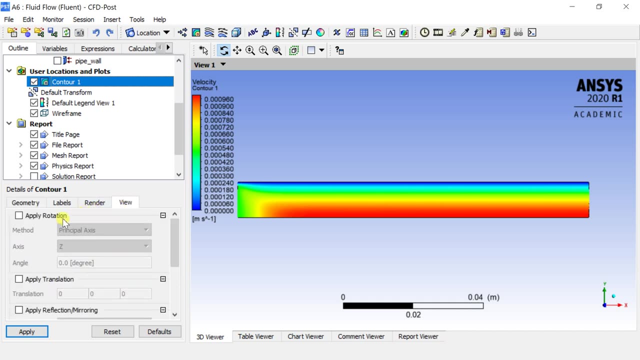 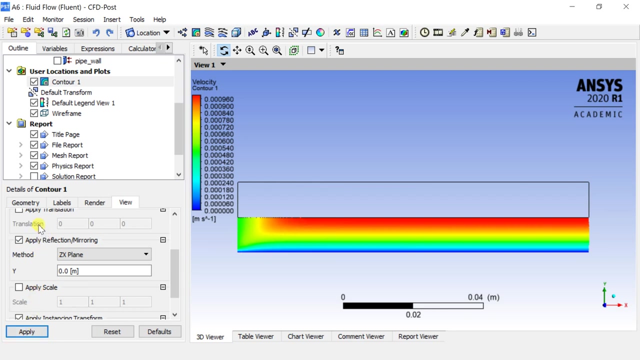 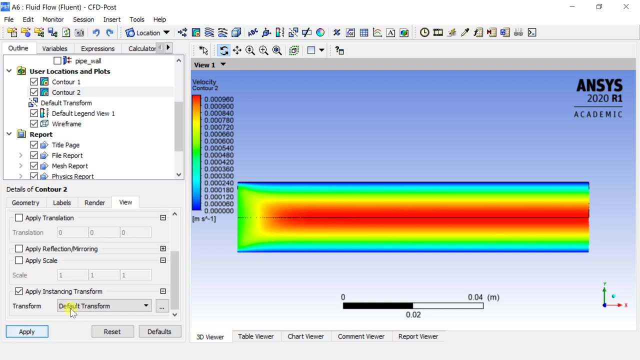 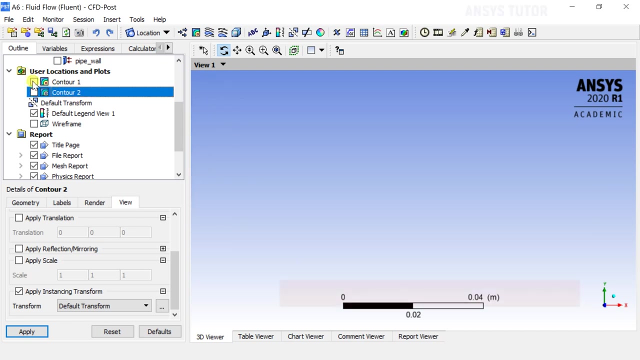 Press I To reopen a première page, The adequacy time. Press I to show the contour for the full pipe body. you need to apply reflection to the contour now. let's create the velocity vector for the domain. add the gradientner to theotz, especially the right Batur. 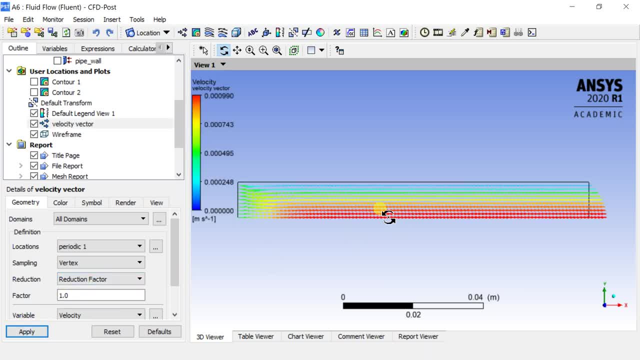 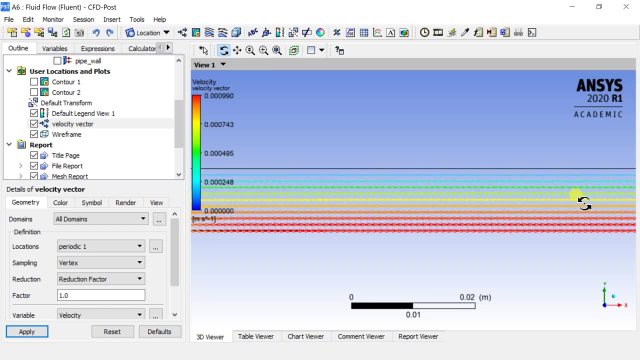 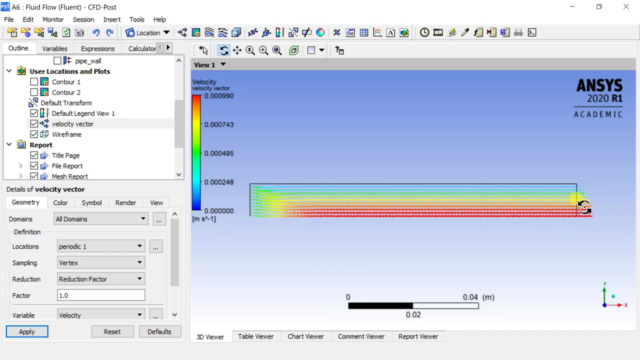 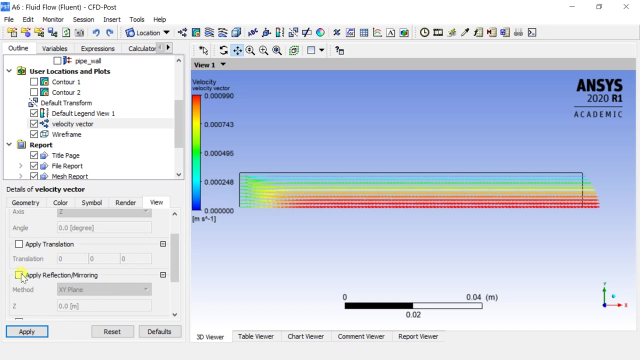 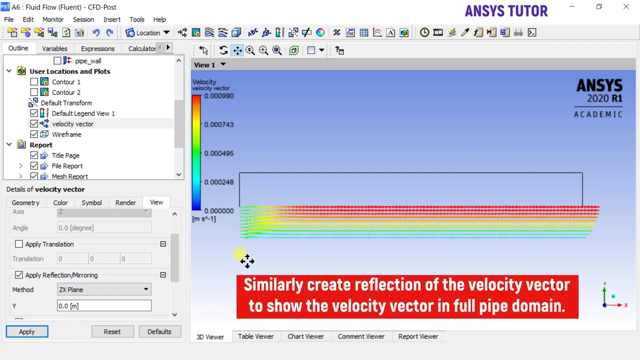 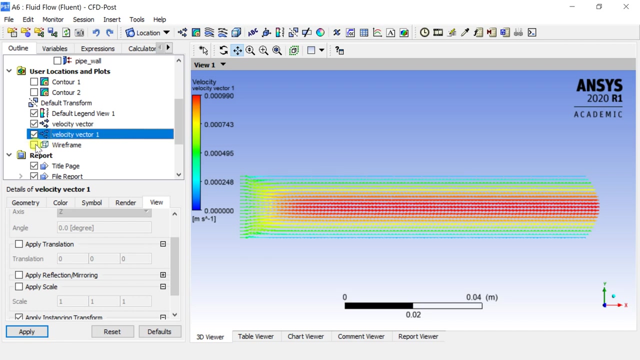 add a few minutes of the rectangle to create the gradient. add an round shape for the rotation. Similarly, create reflection of the velocity vector to show the velocity vector in full pipe domain. You can also modify the velocity vector symbols and sizes. We prayed that you would like to play puzzle with this model also. 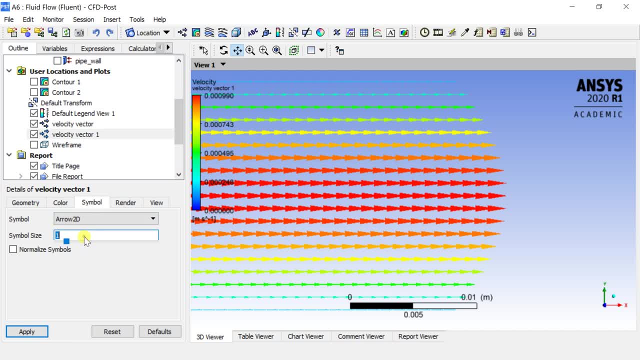 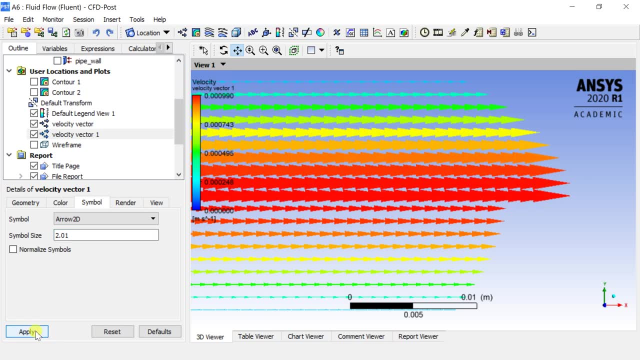 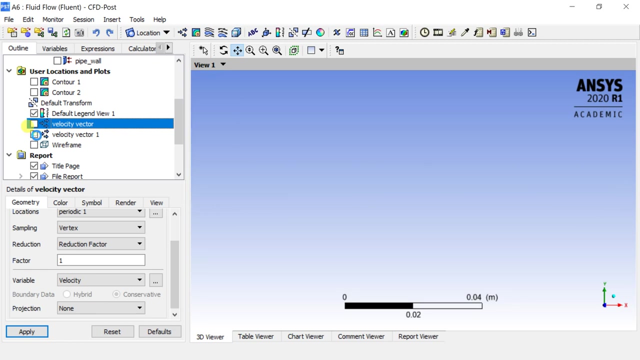 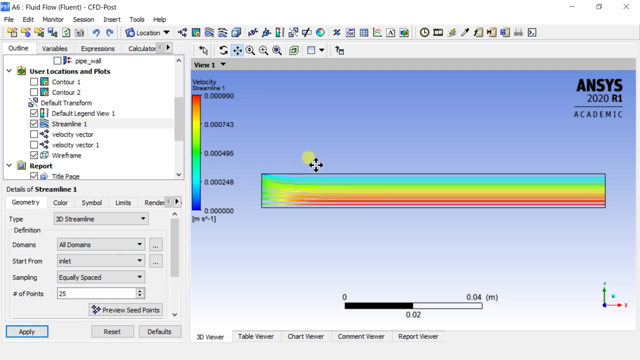 Jump to next video to understand how to play with theifteriamo in full pipe. よって undertera. We pray that you can watch until the end of this video. Bye, byeartz, Let's check the streamlines. Let's check the streamlines. 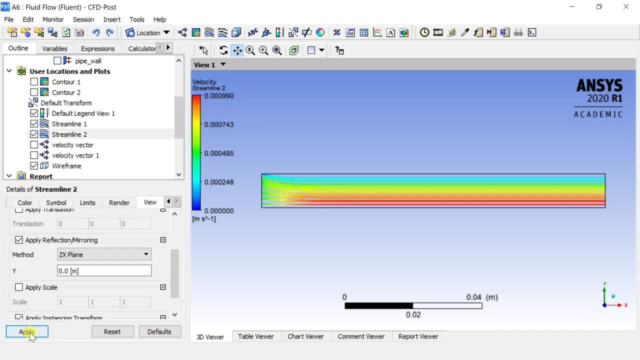 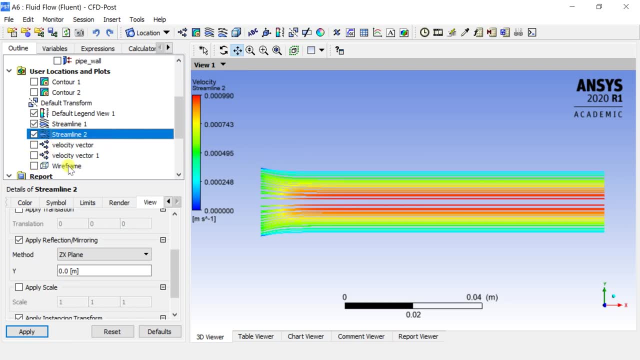 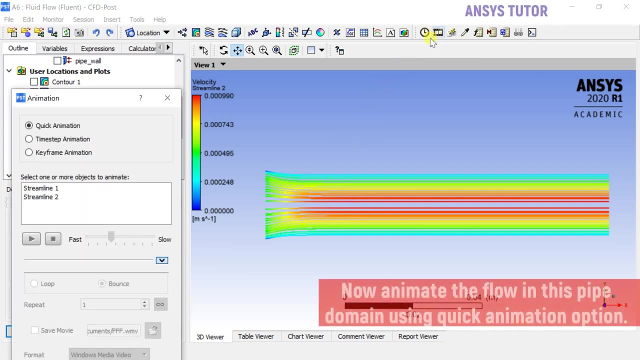 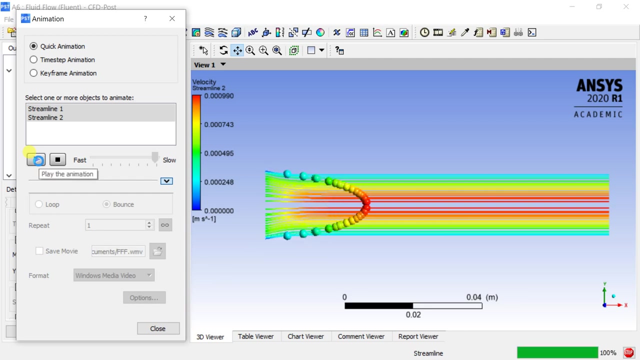 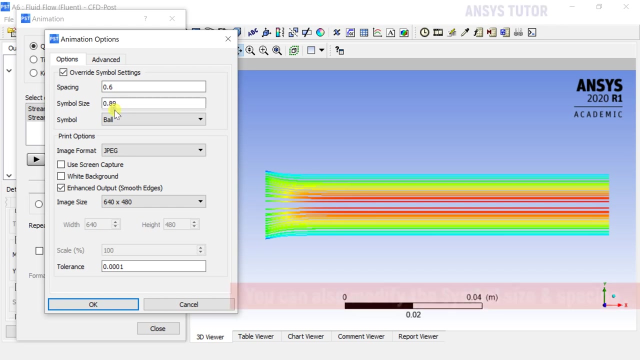 Let's check the streamlines. Now animate the flow in this pipe domain using quick animation option. Now animate the flow in this pipe domain using quick animation option. You can also modify the symbol size and spacing. You can also modify the symbol size and spacing. 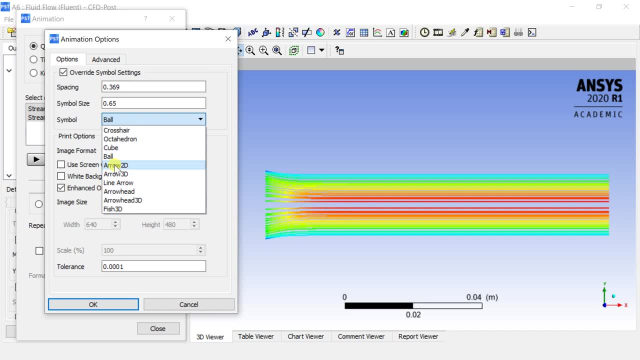 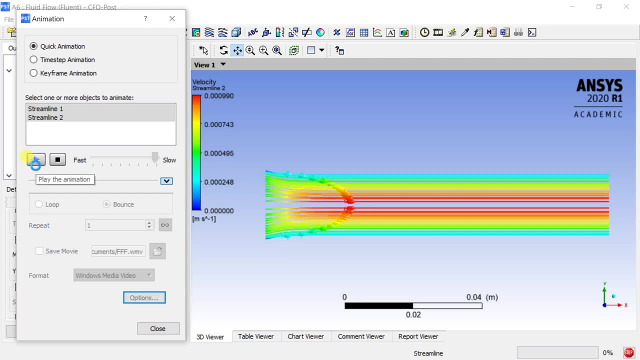 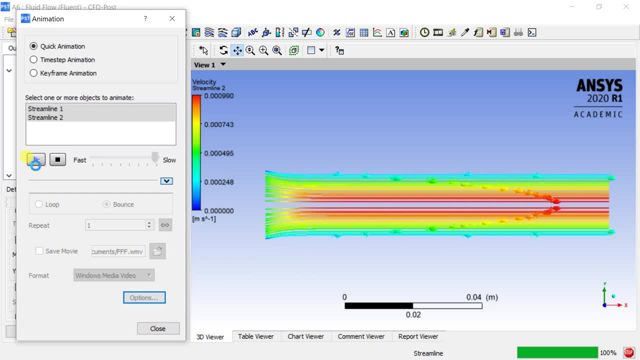 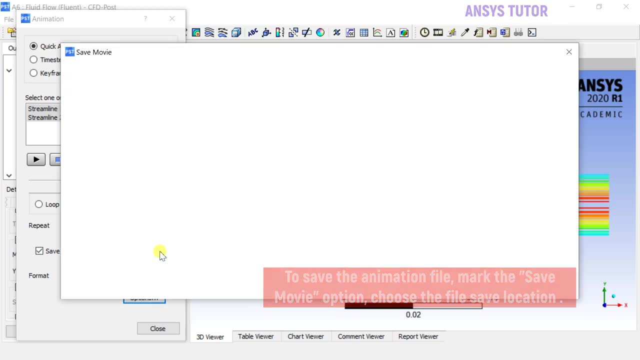 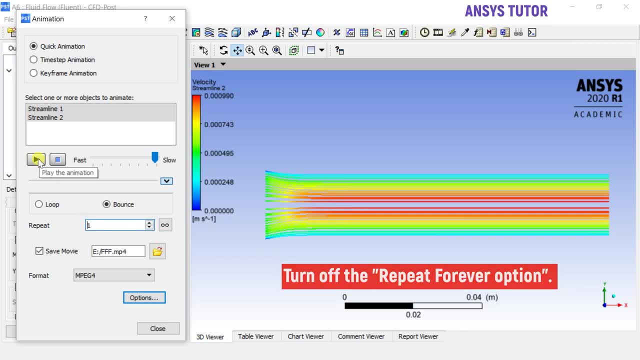 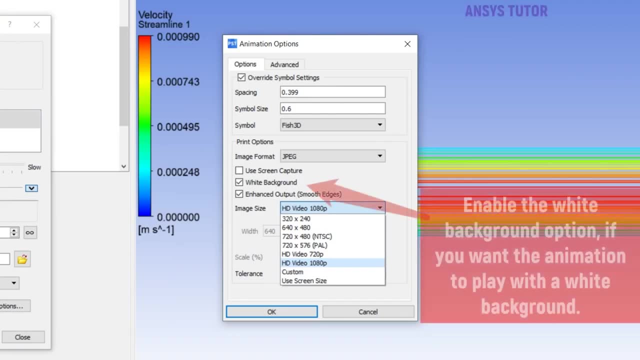